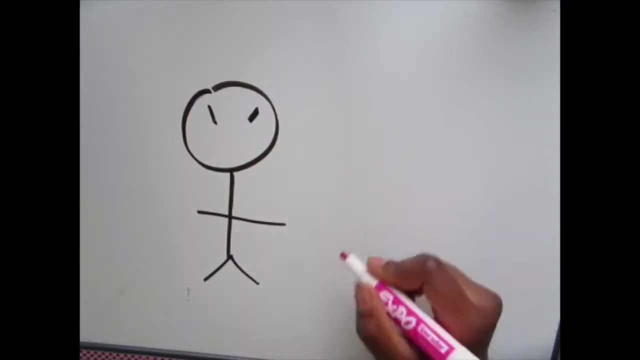 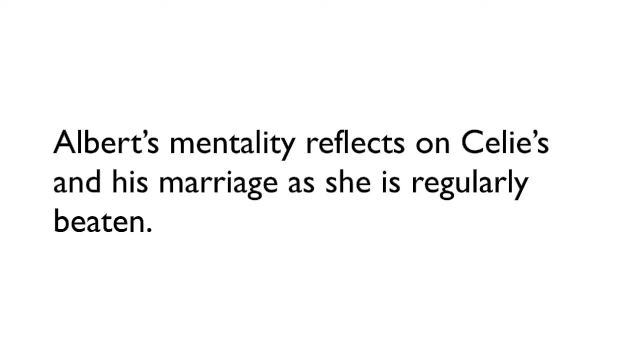 he says, is making them seem inferior and implying that they can be ordered around by the dominant person, meaning the one with more power, which would be the husband in this case. Albert's mentality reflects on Celia's and Albert's marriage, as she is regularly beaten. 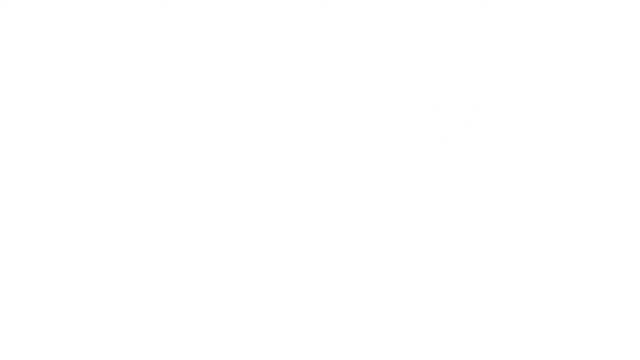 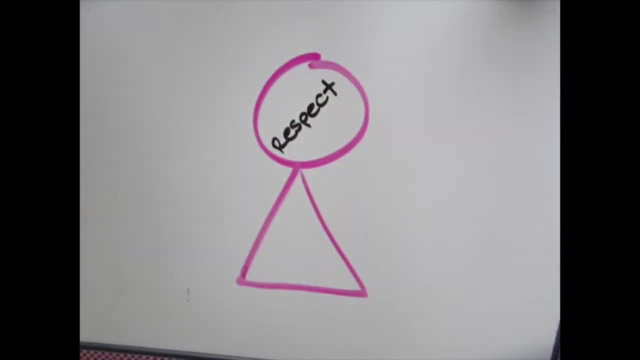 Men such as Albert expect to be the dominant spouse in a marriage, and they think the only way to attain this status is by abusing their wives. This shows the lack of respect women receive in a marriage because of the society's expectations of how a man is supposed to treat. 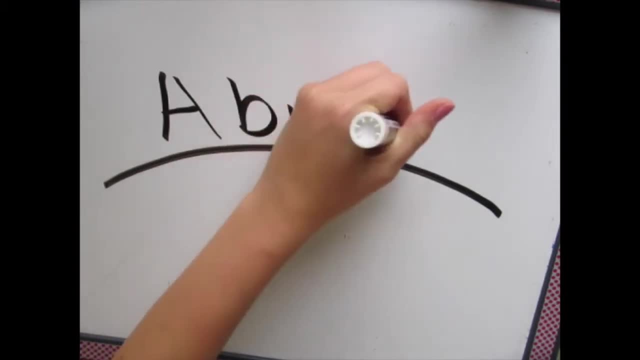 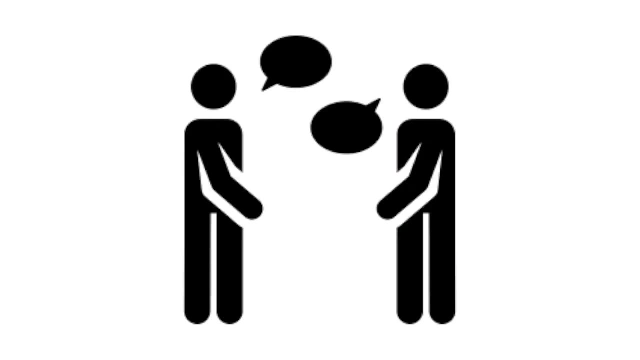 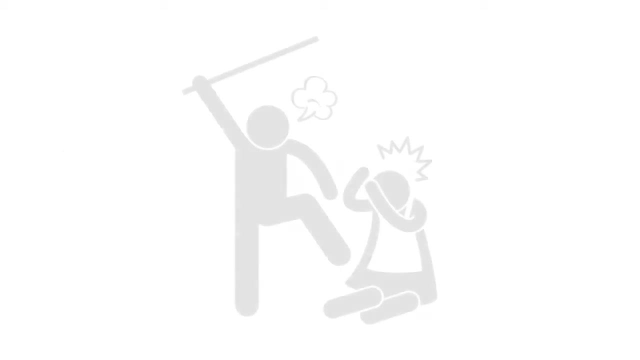 his wife. We see this mentality creating a line of abuse that is carried out in Sofia and Harpo's marriage. While Harpo and Celia are talking, on page 36, he asks her what he ought to do to make her mind. She responds: beat her. Harpo takes her advice. 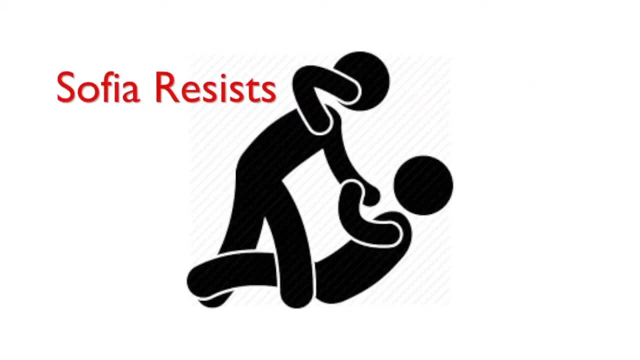 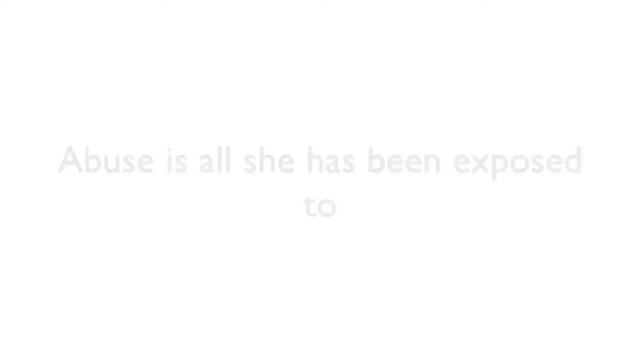 but Sofia resists this oppression and beats Harpo back. Celia initially gives Harpo this advice because abuse is all she has been exposed to in her relationship with Albert. Sofia's response to Harpo's beating is not something that is expected for a woman to do, based on society's 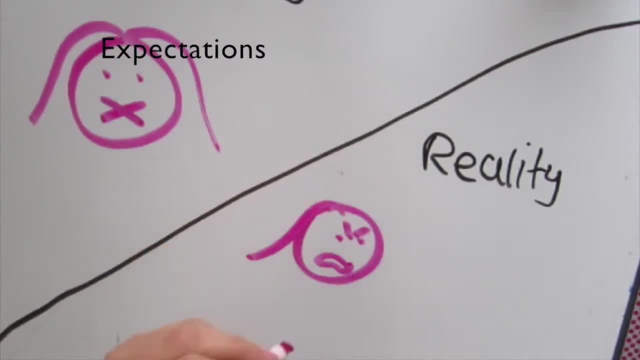 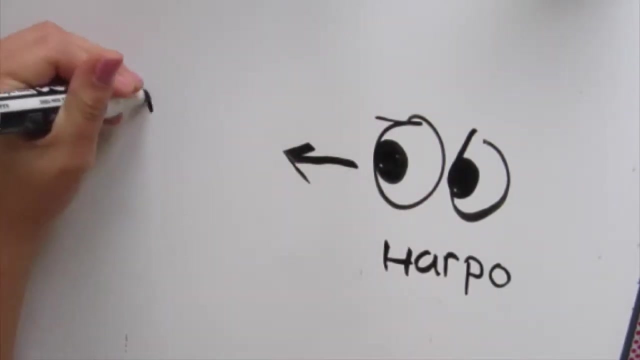 expectations, which are for a woman to silently take a beating. This exemplifies how Sofia defies society's expectations. Sofia is able to do this because of her strong personality. The cycle of Sofia and Harpo beating each other is created because Harpo follows an example from 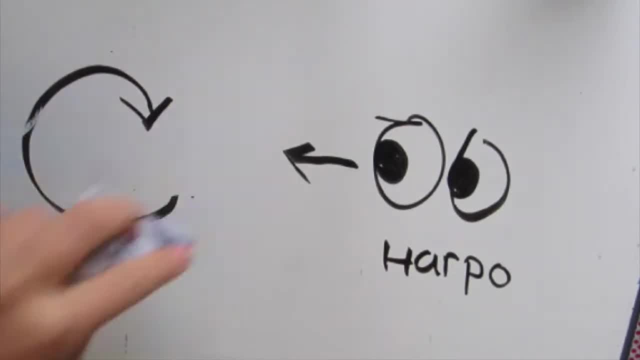 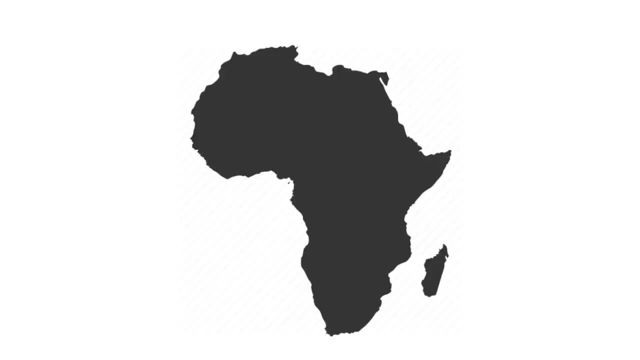 his father. Harpo expects a relationship like his father, where the man is dominant and the woman is dominant. This is a cycle of Sofia and Harpo beating each other. This is a cycle of the man's orders and takes his beatings. In Africa, Nnedi also experiences sexism and sees 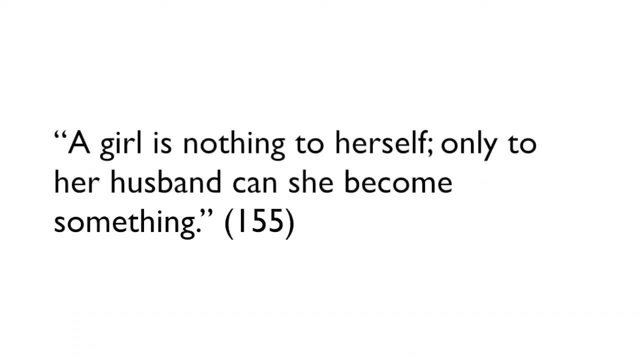 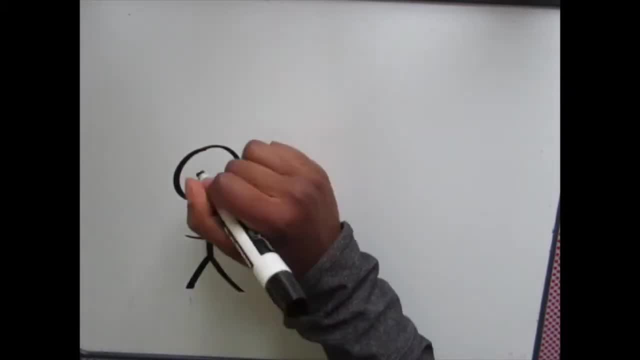 how it is influencing the Alinka people. An Alinka mother says to Nnedi: a girl is nothing to herself, only to her husband can she become something. Through this quote, we can clearly see the role that women play in the Alinka society. Women's only significance is in relation to a man. 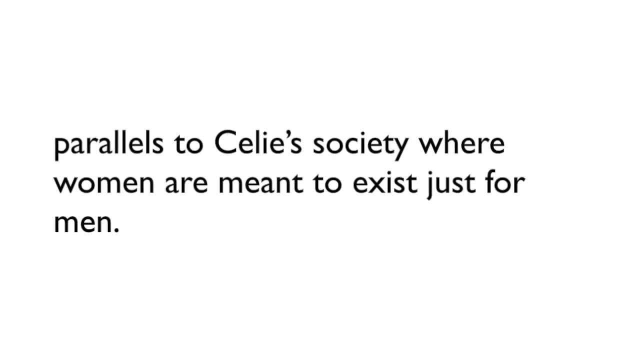 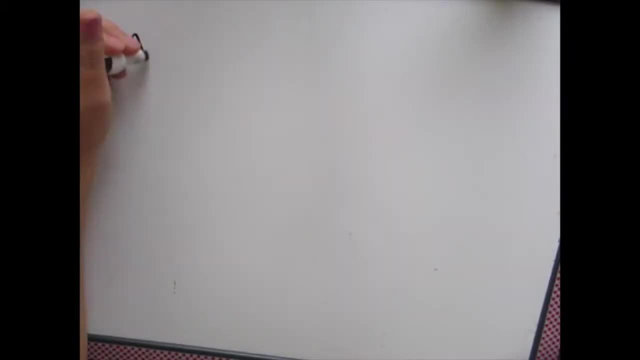 Women do not have an identity of their own, which parallels Cecilia's society, where women are meant to exist just for men. Sexism and racism sometimes pair up to negatively affect the woman of color. in the novel, On page 85,, while Sofia is out with her children, the mayor's white wife asks Sofia if she will be. 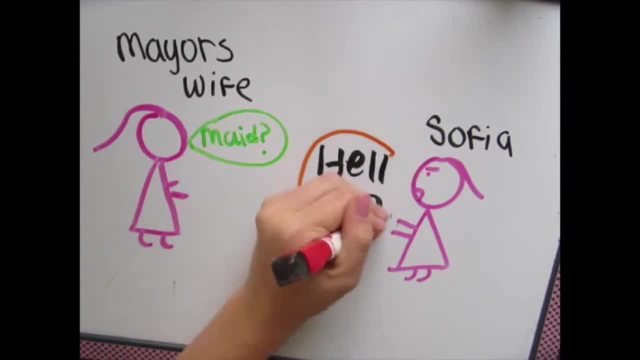 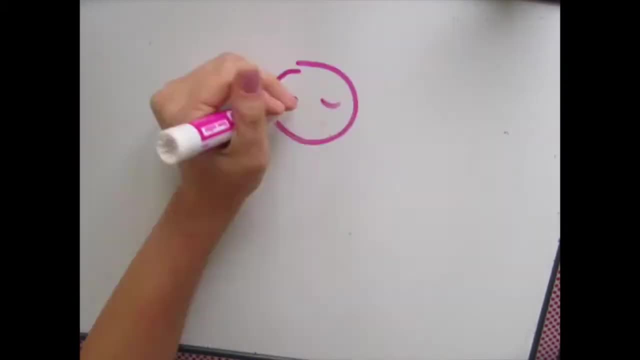 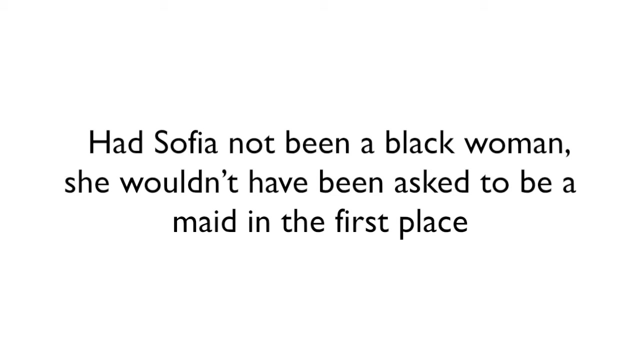 her maid. Sofia responds: hell, no. The mayor then intervenes and slaps Sofia. Quote: Sofia knocked the man down. The police end up beating Sofia and taking her away to jail. Had Sophia not been a black woman, she wouldn't have been asked to be a maid. 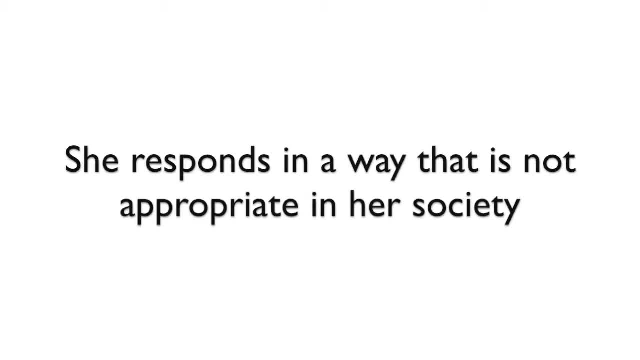 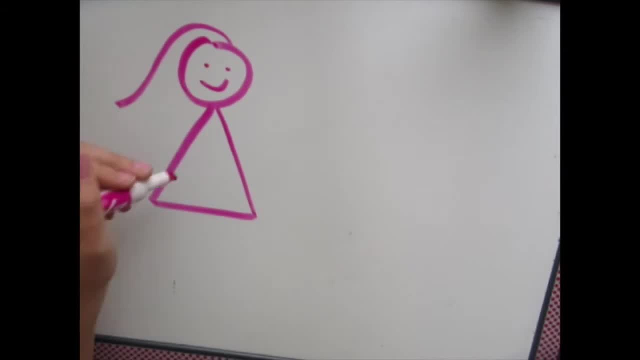 in the first place. She responds in a way that is not appropriate in her society and, as a result, she is abused. She not only got sent to prison for many years, she ended up as a maid for a white woman. This reveals that only after one act of violence towards a white person, a person of color, 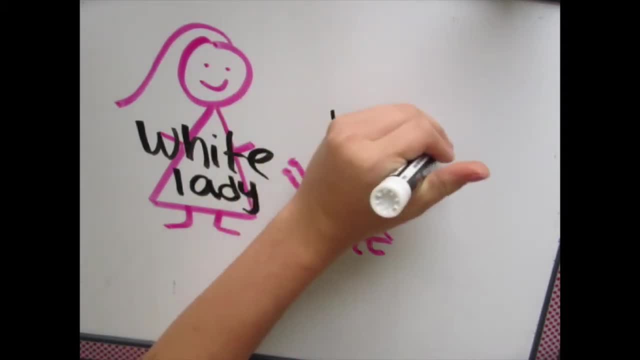 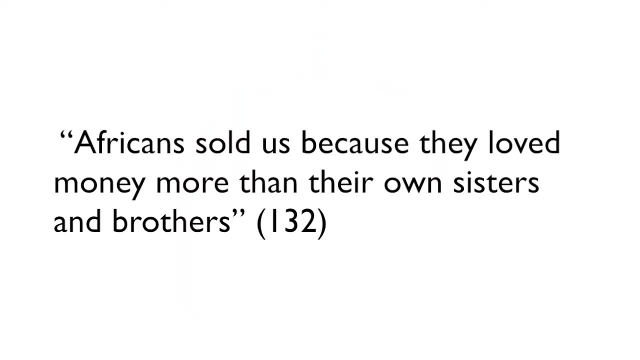 will forever be in debt to them, as Sophia is to Mrs Millie When Celie first reads Nettie's letters. Nettie explains how Africans sold us because they love money more than their own sisters and brothers, showing how they are considered inferior and forced to work For so. 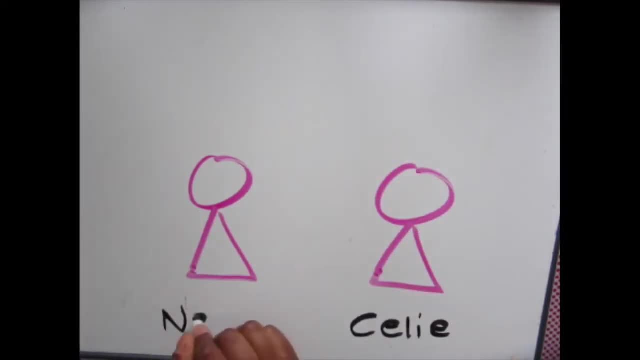 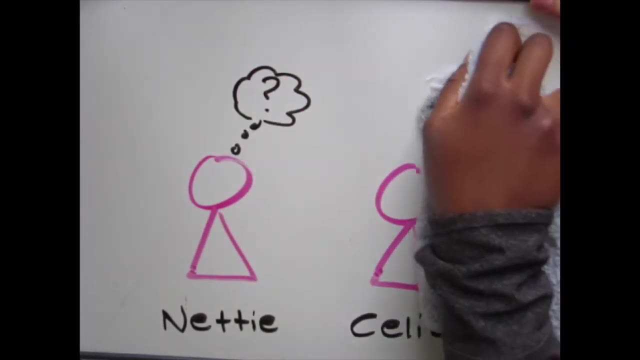 long Celie and Nettie have lived in ignorance about how they ended up in the positions that they're in: Celie being a child wife and abiding to whatever Albert says and not knowing why she is forced to do this, Nettie starting in the same position. 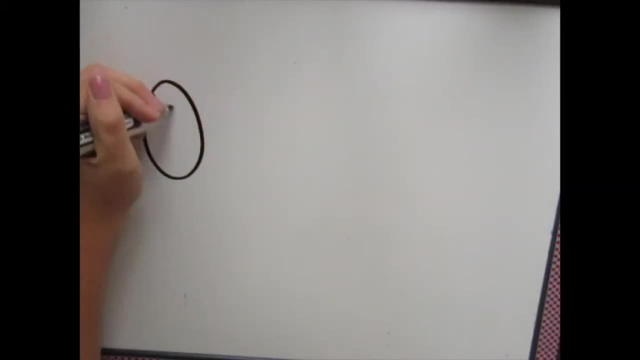 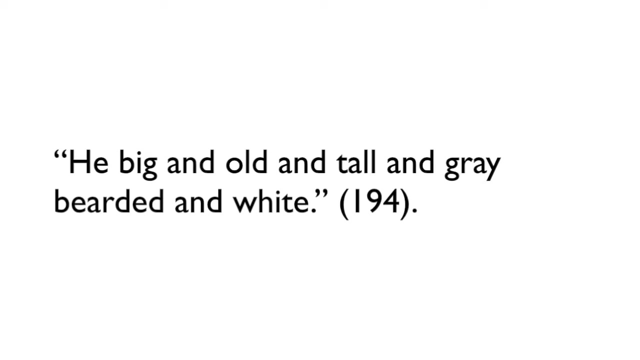 African-American criticism is also seen when Celie explains to Shug her idea of what God looks like in her eyes. Celie explains that quote: he big and old and tall and gray bearded and white, page 194.. The fact that Celie imagines God as a white man exhibits that because white people are 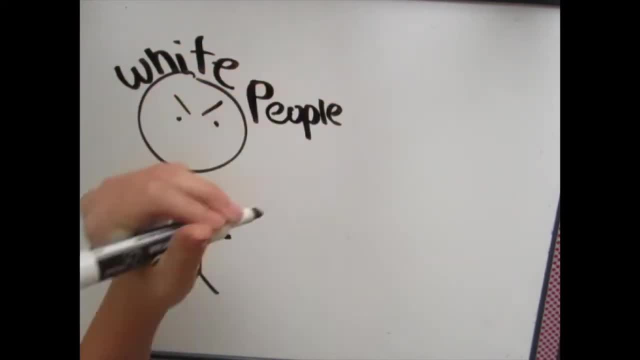 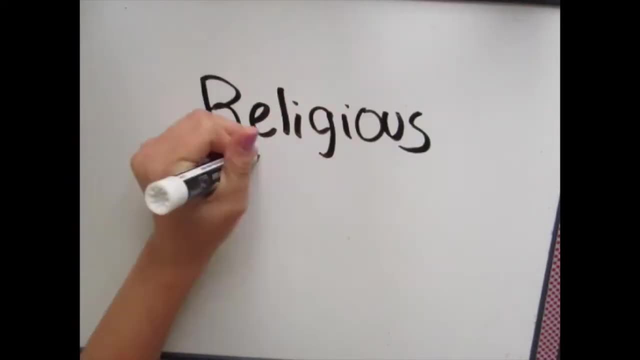 considered the dominant race. this mentality is not only practiced in everyday life, shown by Sophia's example, but also in her own life. Celie explains that quote. she is not only an example when she is beaten up by a white man, but it is ingrained in religious and spiritual 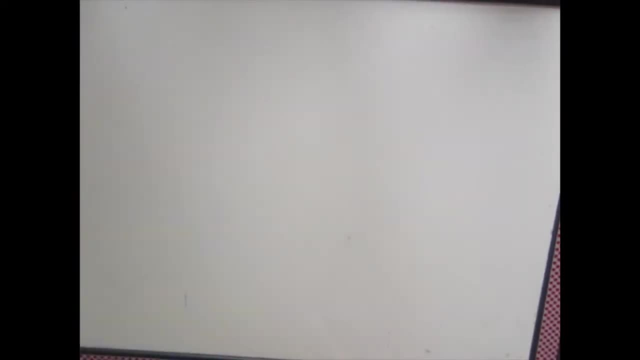 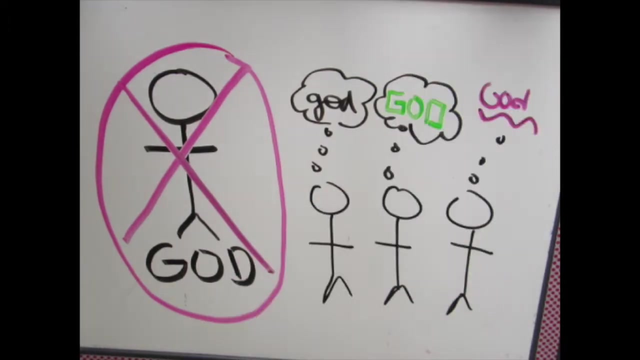 beliefs as well. Celie envisions this idea of God being a person, a person who, in her life, would act as her oppressor, a white man. Shug, attempts to explain to her that God isn't a person, but a being that is interpreted differently in everyone's eyes. Celie then discards her view of God and 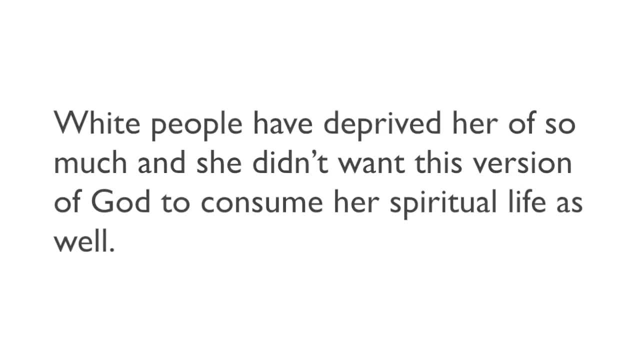 changes her interpretation. She realizes that white people have deprived her of their rights of so much, and she didn't want this version of God to consume her spiritual life as well. Through African-American criticism and feminist criticism, we are able to further understand the